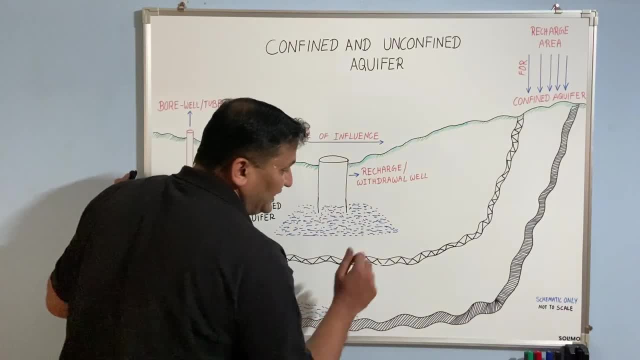 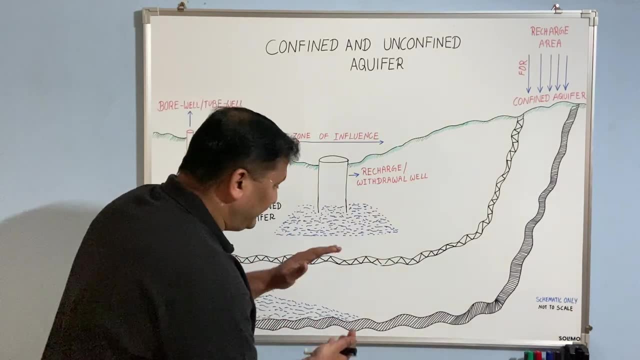 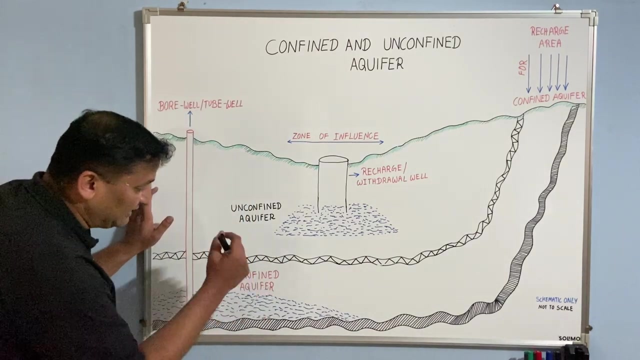 layers. As the name suggests, there are two layers. It can be either clay, rock, shale or anything, And if the water formation is there between the confining layers, we call it as the confined aquifer. So the borewell goes deep into the confined aquifer and extract. 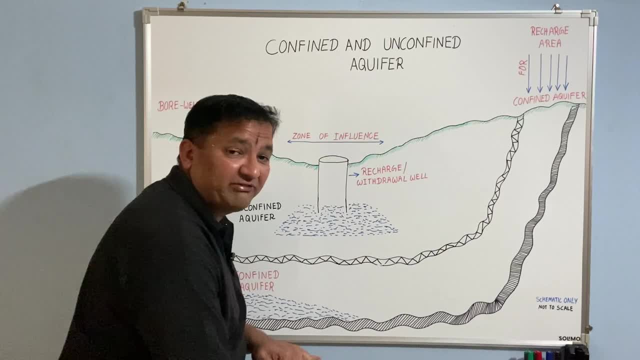 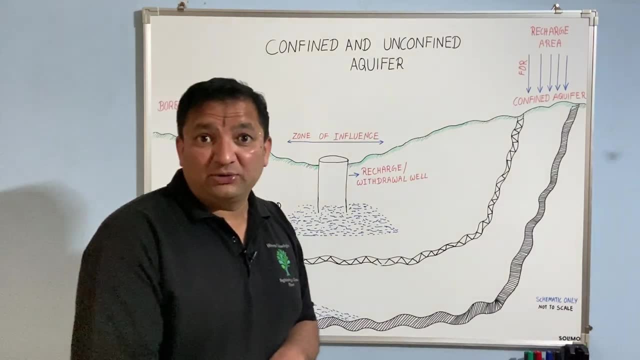 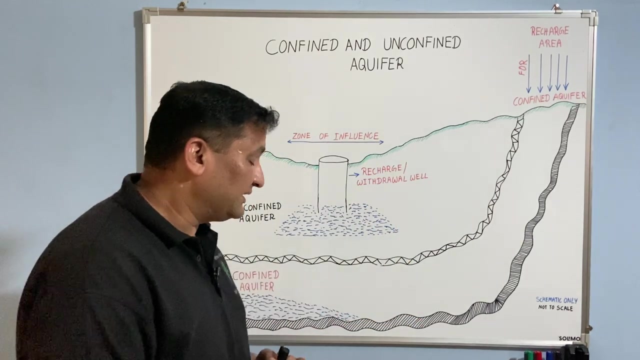 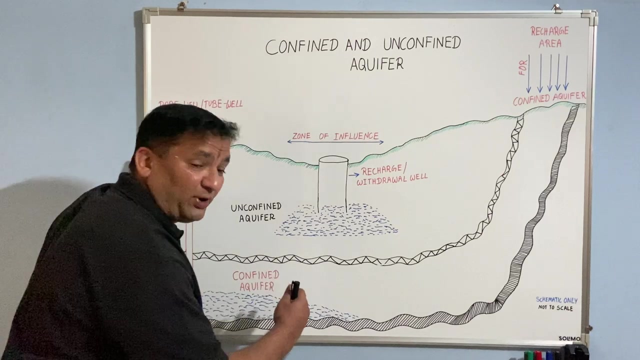 water. Since it is between two confining layers, the water will be greater than the atmospheric pressure Because the water is much deeper into the earth. it will be generally free from bacteriological contamination, But, however, it may contain some chemical contamination. The other thing about the confined aquifer is the recharge. 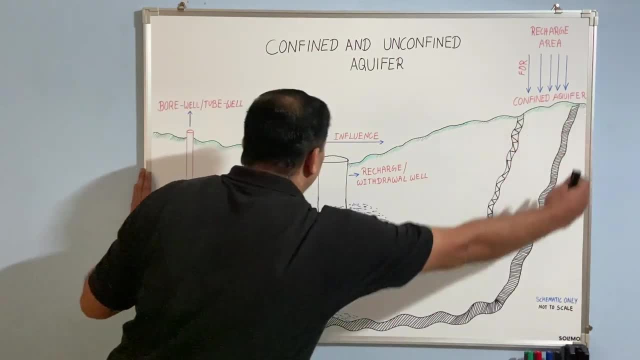 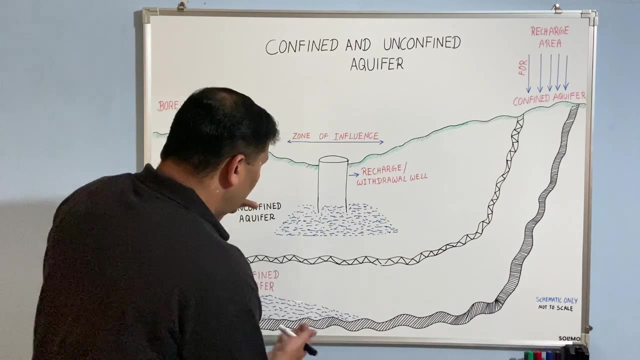 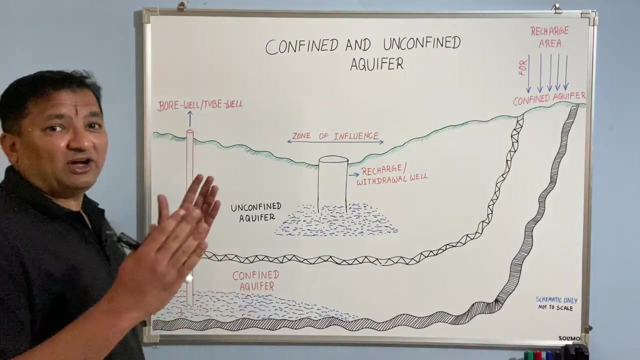 point of this confined aquifer is generally very far away from the source, point of withdrawal, And this formation takes generally decades or even centuries for this water to form between these layers. generally, when we talk about borewell or we talk about groundwater, people are most generally 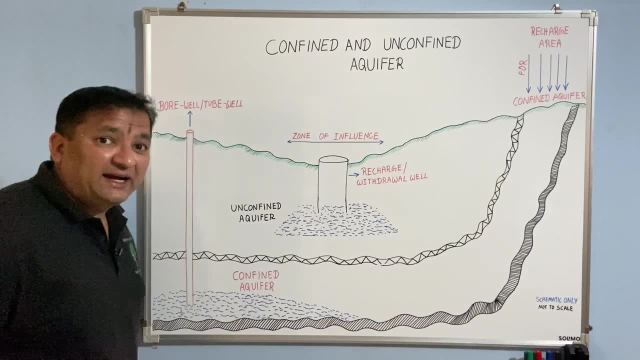 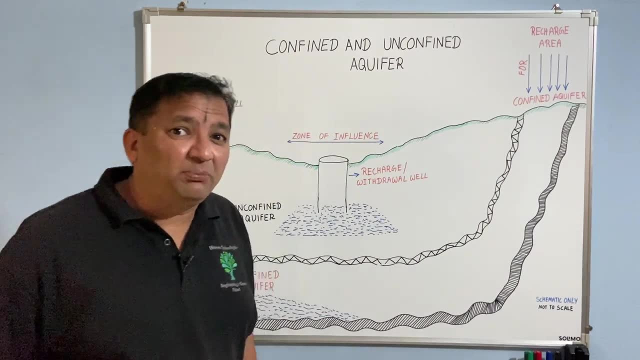 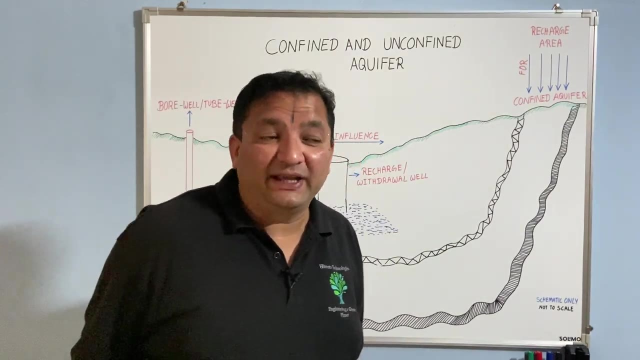 referring to what is called as the borewell, going into the confined aquifer. however, there is one more aquifer which is becoming slightly popular now, called the unconfined aquifer. say, about three or four decades back, no one would have heard the term borewell. the borewell was introduced to. 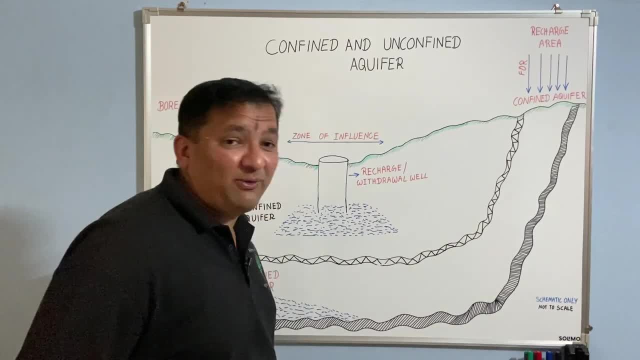 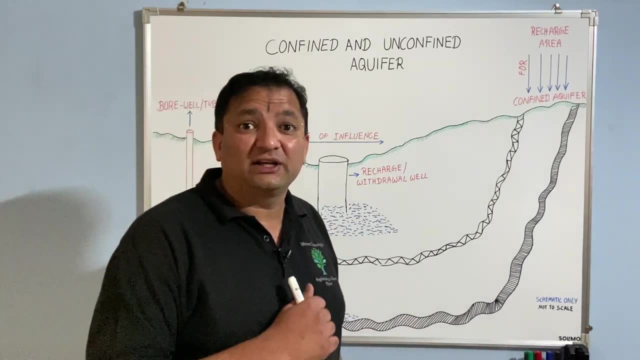 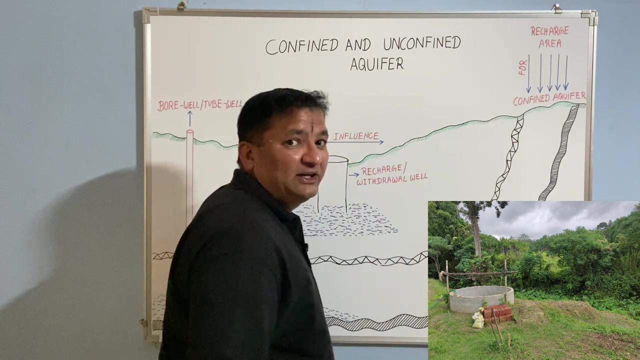 India in the late 1960 by UNICEF, and I was told that the first borewell rig is still preserved somewhere in Pune, say about 30-40 years back. when people spoke about groundwater, they were essentially referring to an open well. an open well is a well which is drilled into the, or rather, 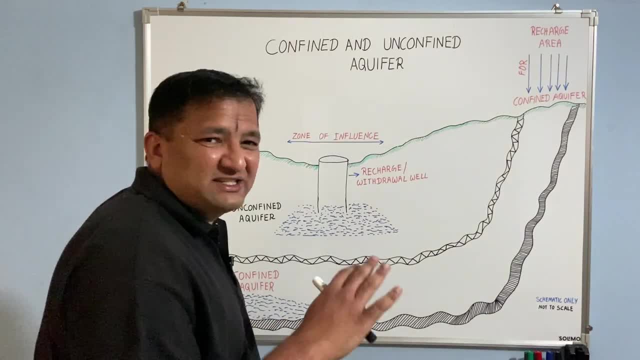 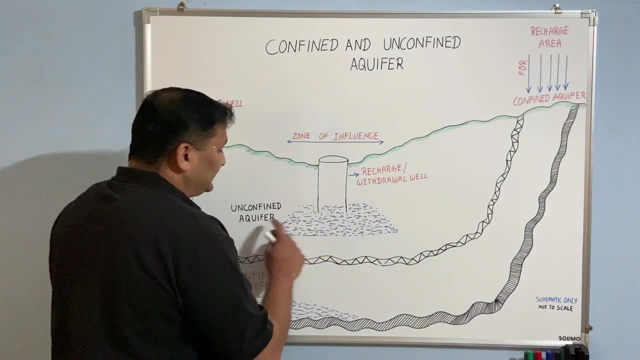 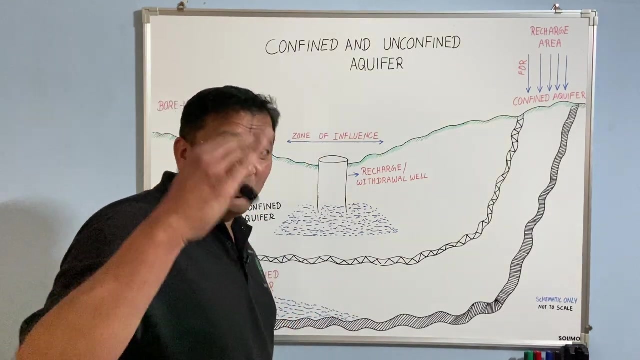 which is made or sunk into the earth, which is generally not more than 30 or 40 feet, sometimes even lower than that, and when that well hits the water, this water is called the unconfined aquifer. this is at atmospheric pressure, so one can actually see the water level going up and down. 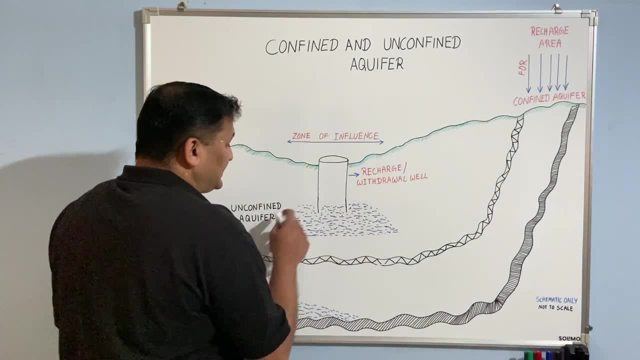 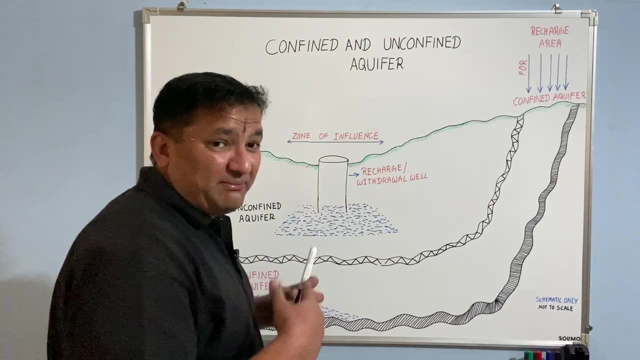 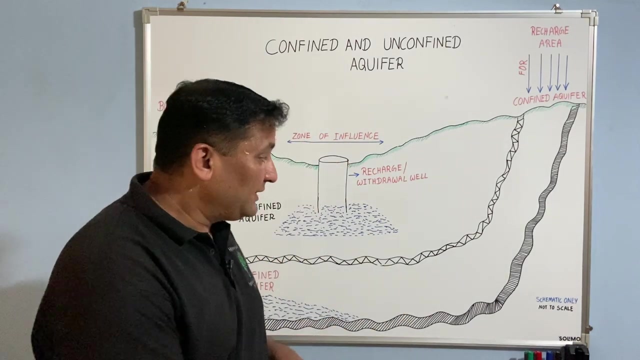 through the course of the year. so this is the well which taps into an unconfined aquifer. depending on the space and environment and the surroundings, there may be some chemical contamination or bacteriological contamination in this unconfined aquifer or the shallow water. however, in most cases, 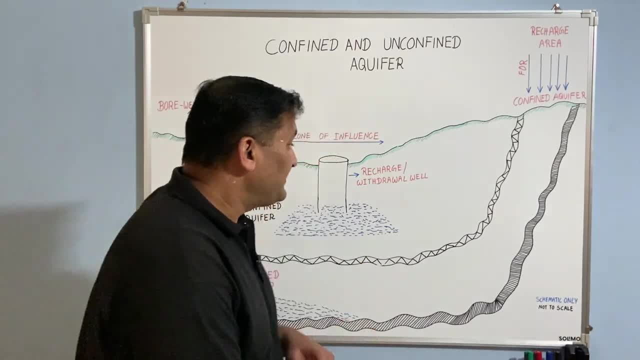 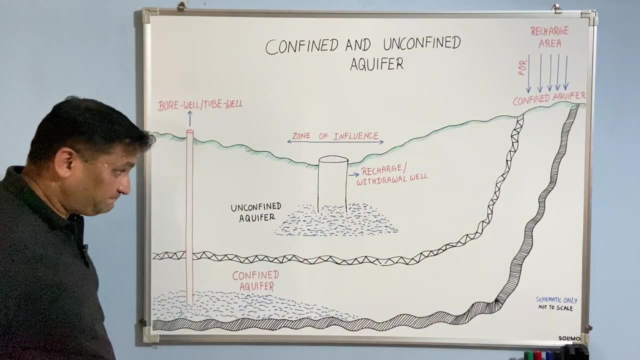 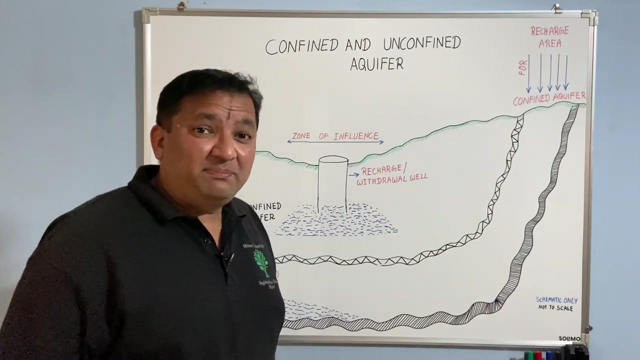 it will be free from chemical contaminations. so this is the well which is being drilled into, the, and the depth of the well is far, far, far lower in comparison with the deep borewell, and this depth is generally 20-30 feet, not more than that in the urban context when people say that you know there. 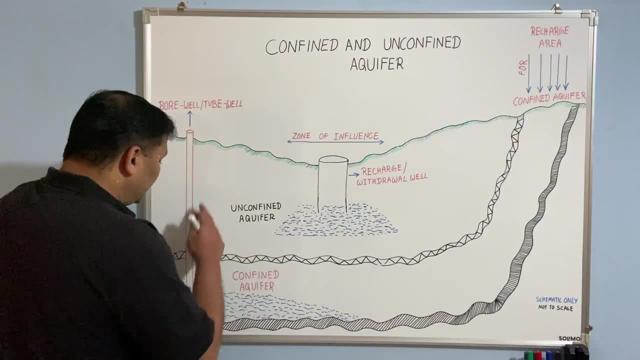 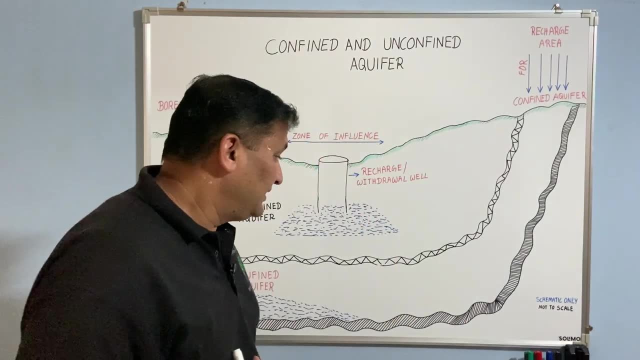 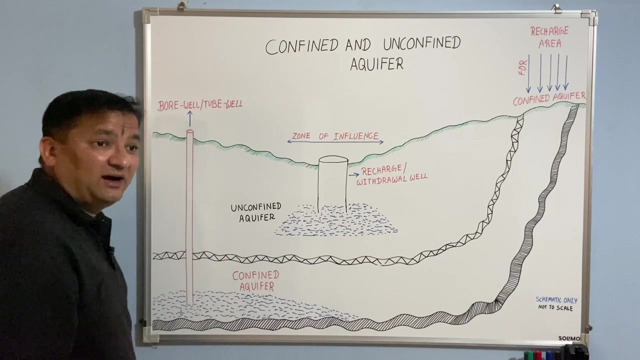 is no ground water. people are generally referring to no water in the borewell because people are almost forgotten about the concept of an open well or a shallow aquifer well, but there is a very good chance that the chance that you know, even though you don't find water in the deep, unconfined aquifers. 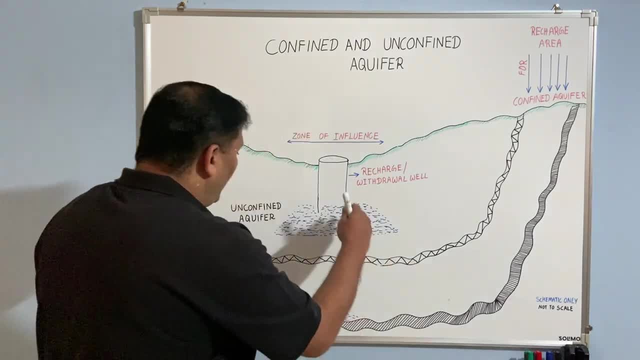 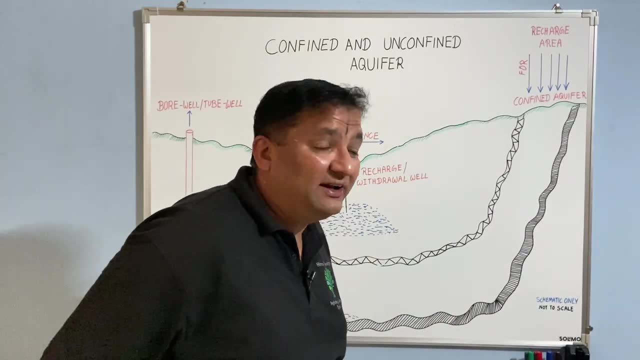 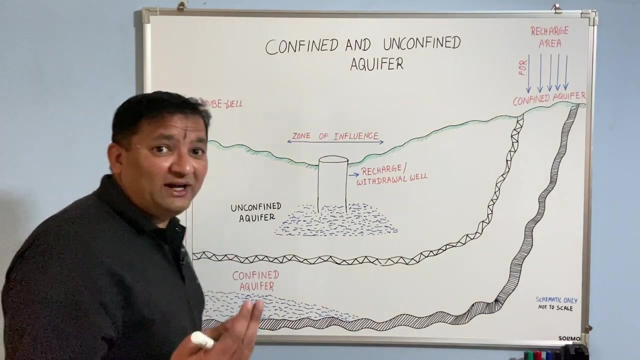 there may be good amount of water available in the shallow well or the unconfined aquifer. From where I am speaking right now, there is a site just about 200 meters away where there is no water, at 1400 feet in the borewell, which is tapped into the confined aquifer, while 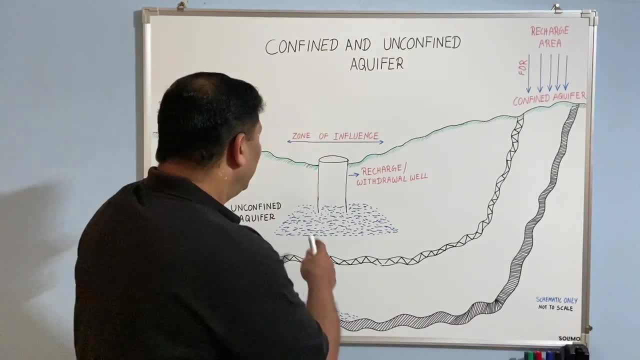 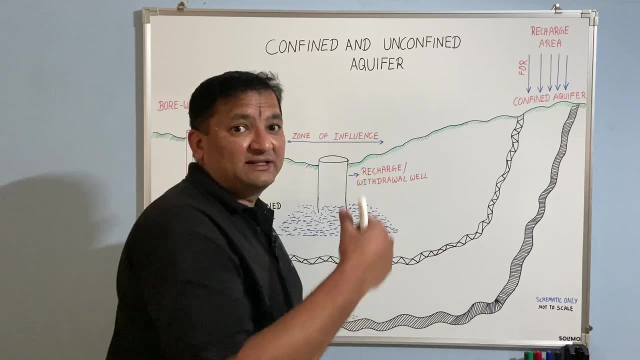 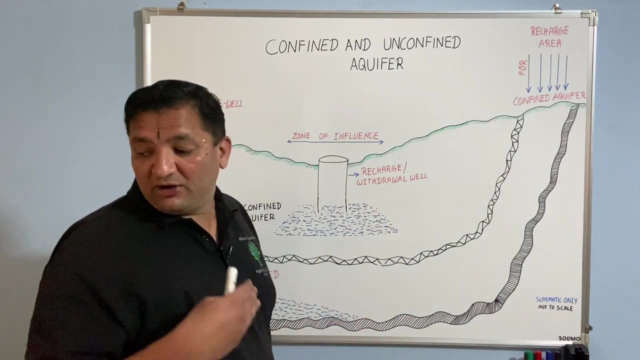 there is good amount of water available just about 10 feet in the unconfined aquifer when we have drilled, or rather we have just sunk an open well or a recharge well. So generally in the urban context we can now try to revive what is called as an open well. 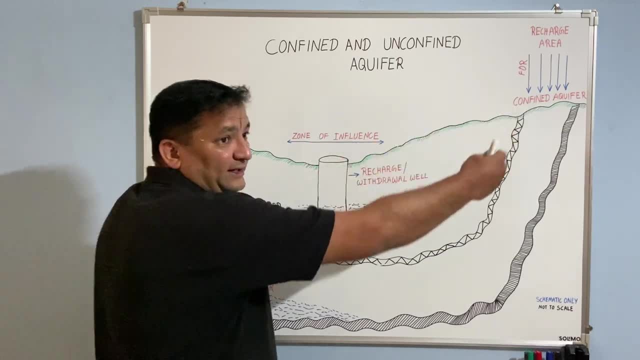 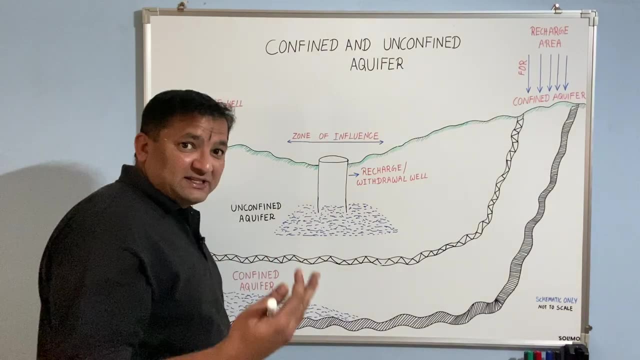 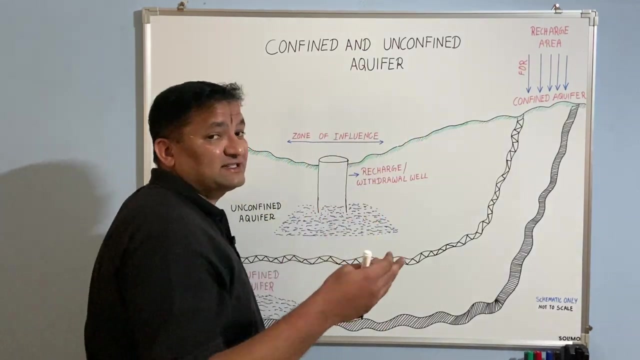 or the recharge. well, try to pick up the water from the rooftops or the roads and push it into the unconfined aquifer for recharge and withdrawal later. In good number of cases, even when we are actually doing the well for recharge, there is chance. 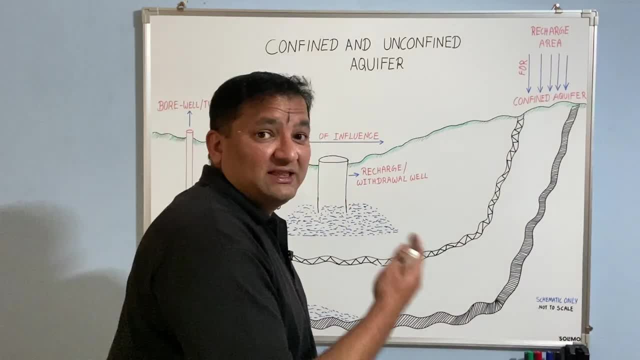 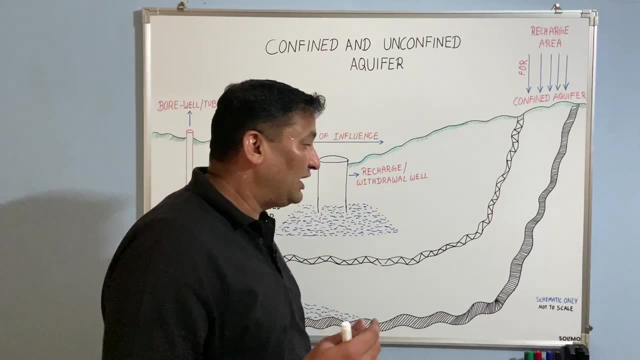 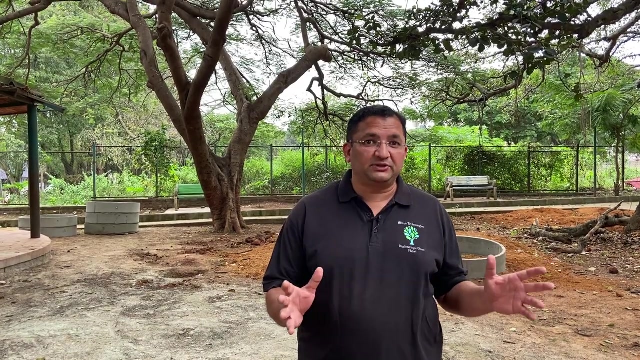 that the water may come back from the same. well, We will now go into the field and see both the borewell and the recharge. well, or rather even you can call it as the withdrawal. well, at close proximity, let us just go right now. We just saw the schematic representation of the two general types of the aquifer: the confined, 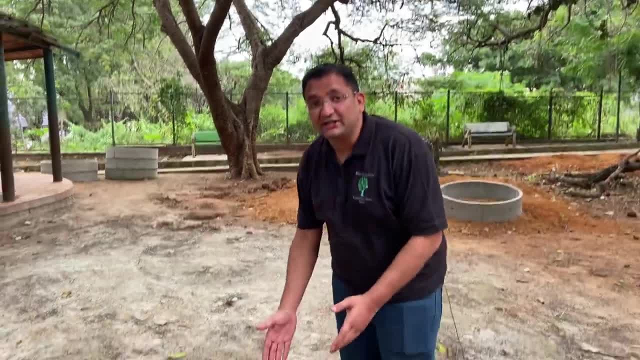 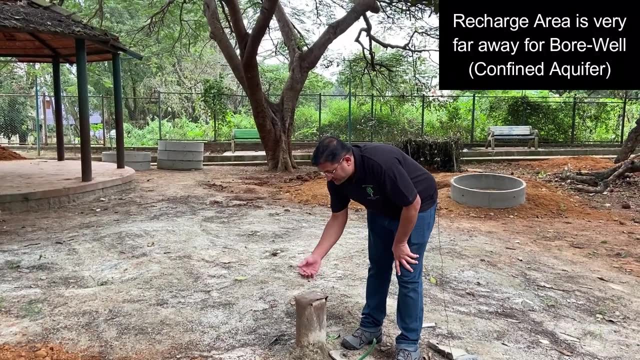 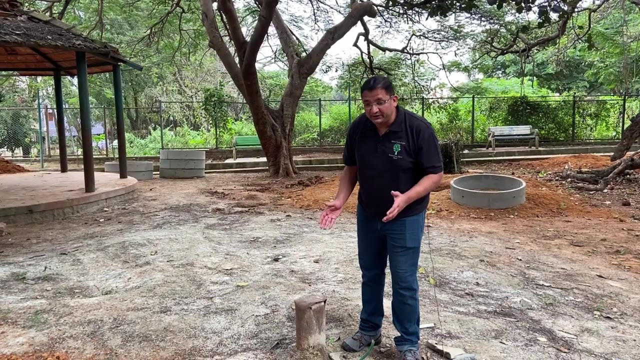 and the unconfined aquifer. So this is what we generally call a borewell. this goes deep into the earth, into the confined aquifer, So the water which comes out of this is under pressure. So this, the kind of wells, that is, the borewells, are very common in the urban context and we 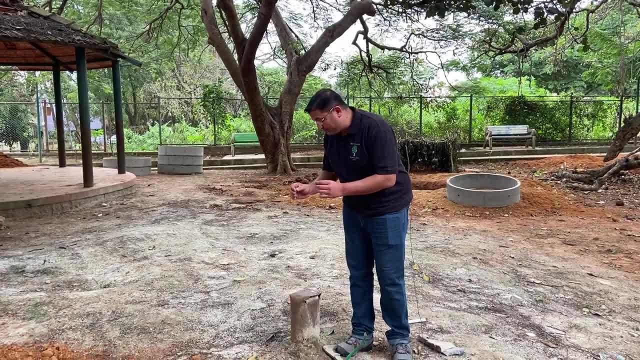 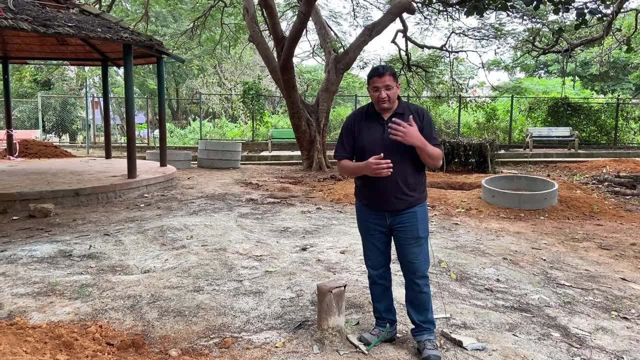 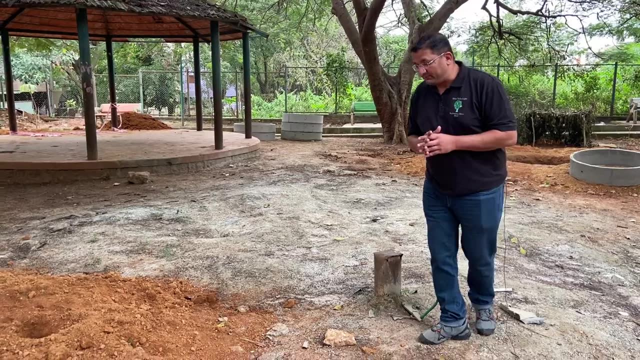 quite often hear that the wells have dried up. that is what they mean is the bore wells have dried up, that there is no water in these kind of bore wells? We have earlier spoken about the recharge wells or the unconfined aquifer, So we can just come here. 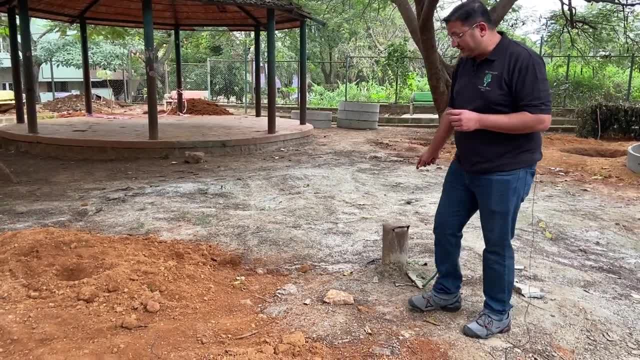 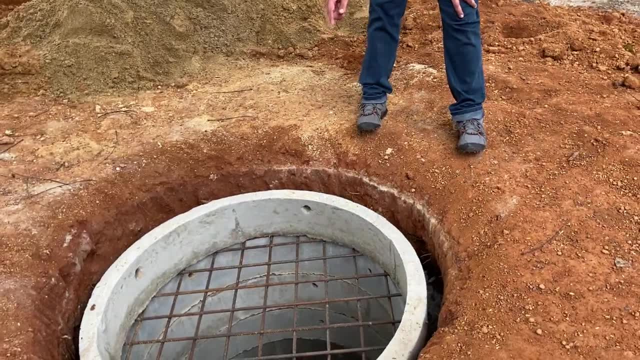 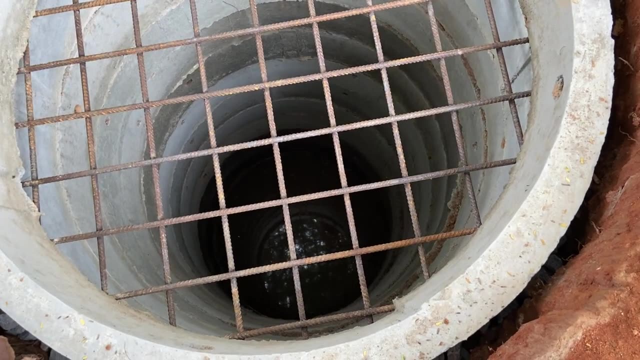 There is a bore well here which goes into the confined aquifer. If I just walk about 10 feet from that borewell, we have a shallow well or a well which goes into the unconfined aquifer. We can see here. the water here is available at just 10 feet. 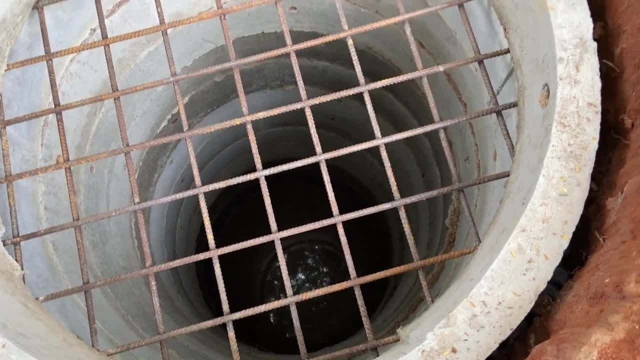 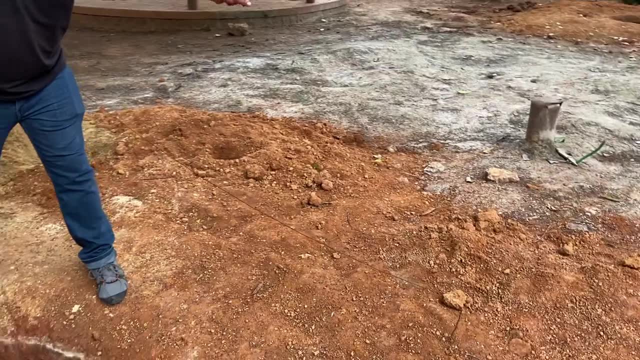 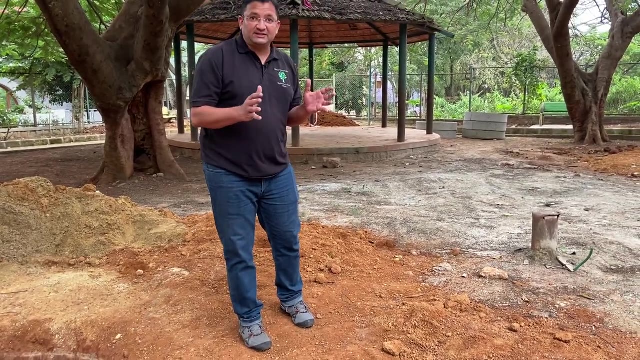 The water here- I am repeating- is available at just 10 feet, whereas in that borewell, which is just 10 feet away from this well, there is no water, even at 1400 feet. So this is essentially The difference between the two kinds of aquifers. in many cases we can find that there is no. 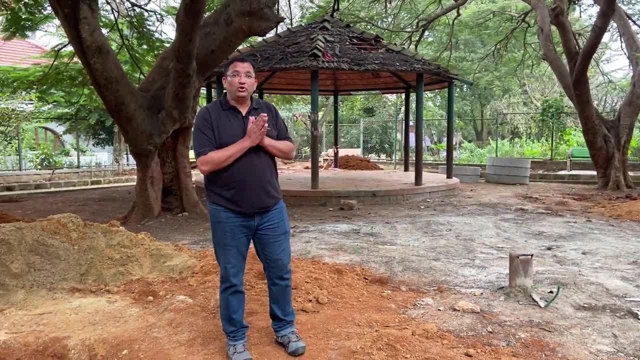 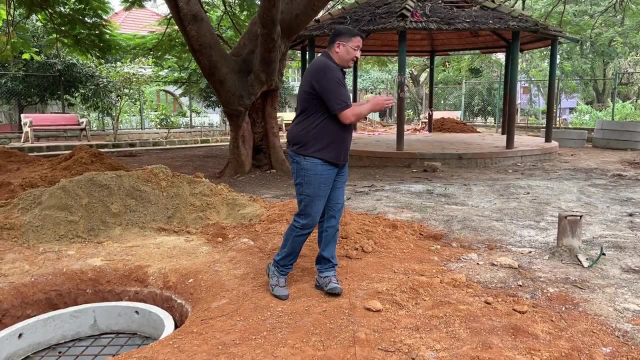 water in the deep well, that is, the borewells. So even if you go to 1500, 2000 feet, there may not be any water in the borewells. that is no water in the confined aquifer, whereas in the unconfined aquifer water may be available. 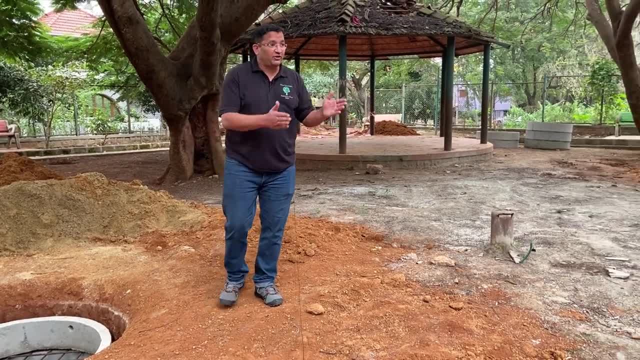 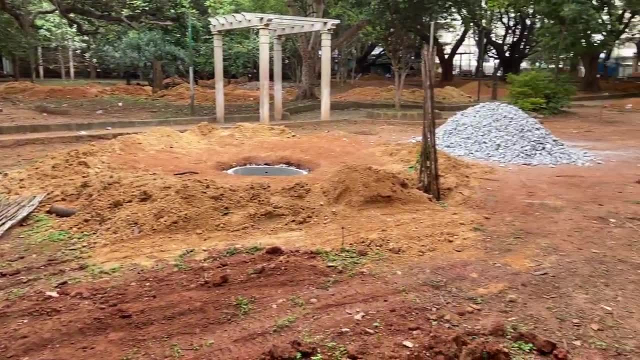 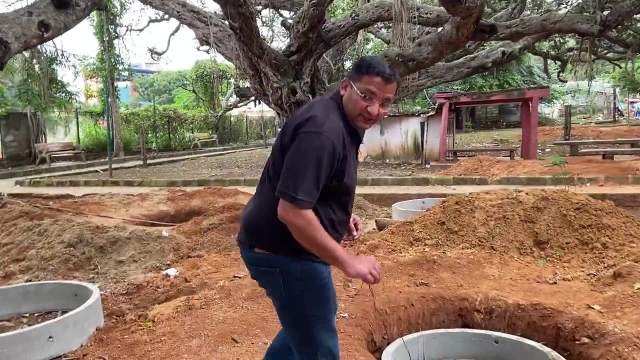 at just 10- 12 feet. You can see this place around. we have got multiple wells here. almost in all the wells the water is available between 10 to 15 feet. You can come here. I will show you one more well: This well, which is again just about 30 feet from that borewell. we can see one more well. 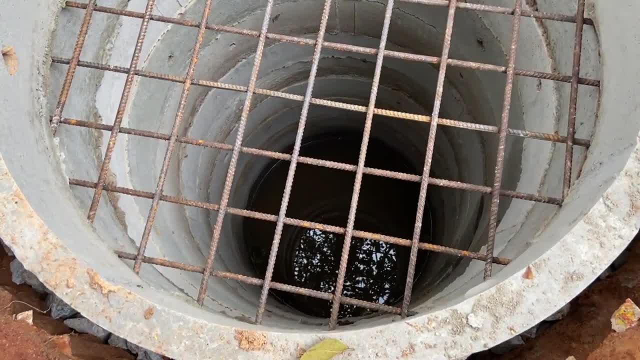 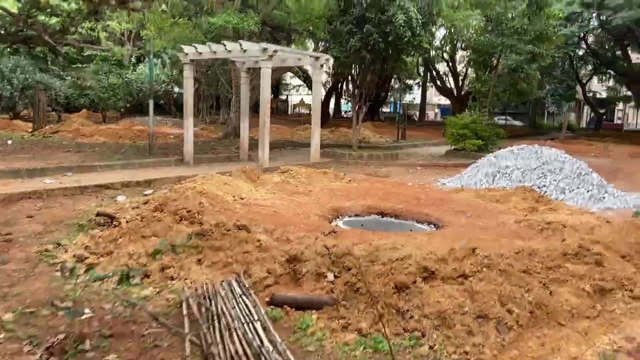 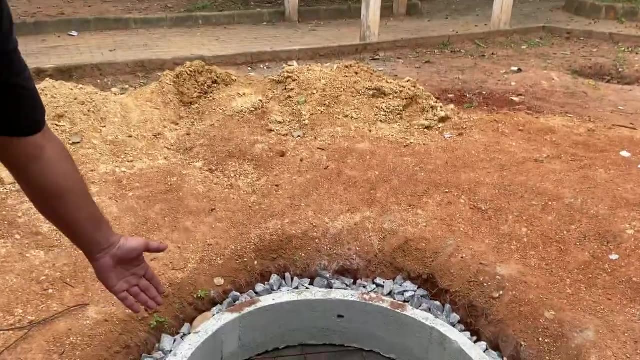 here again. the water here is available at about 12 to 15 feet. There is one more well just about maybe about 50, 60 feet from the borewell. Then in this well you can see, water is available at roughly about 15 feet. 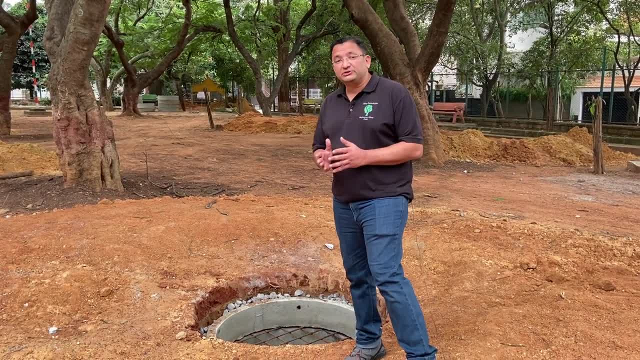 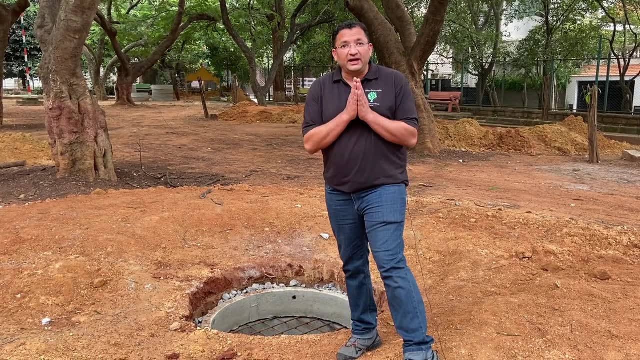 So these are the kind of structures which are useful both for withdrawal as well as recharge. this, what we call as a recharge well, is essentially a small cavity into the earth. in this case, as we saw, we are actually getting water from the well. this can technically be. 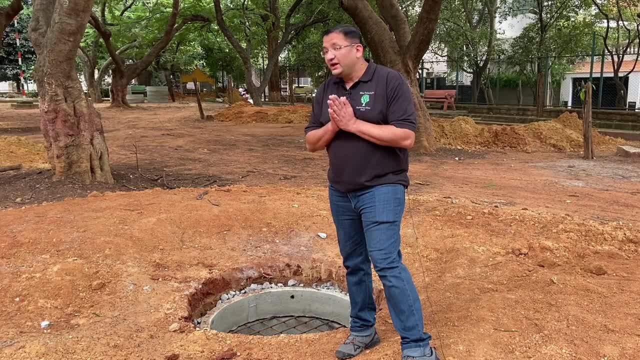 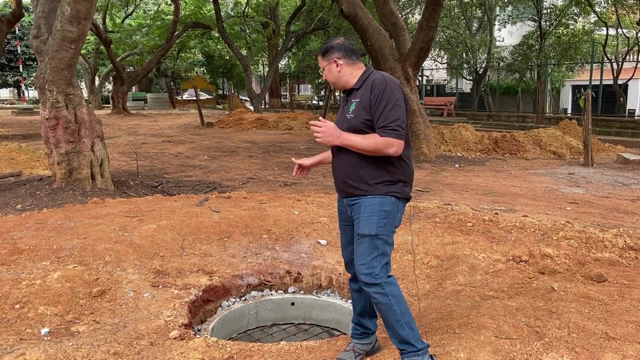 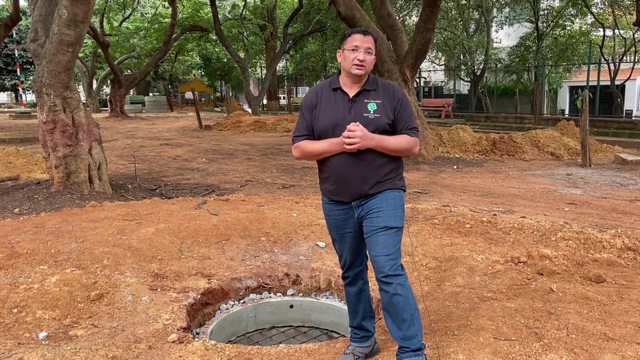 used. We will see how good it is for portable purposes. However, It also can be used to pick up the runoff from the, from the catchment, and that runoff can be diverted into this well for recharge, So the runoff can get into this well and augment the groundwater. 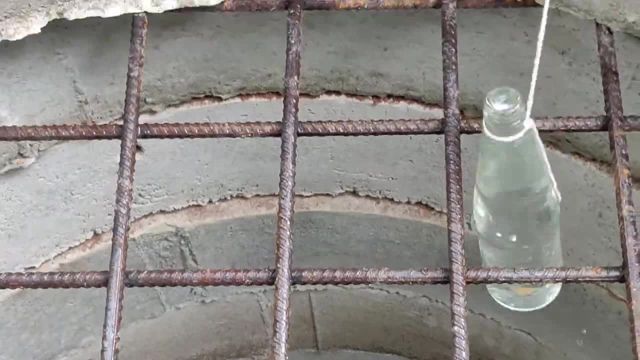 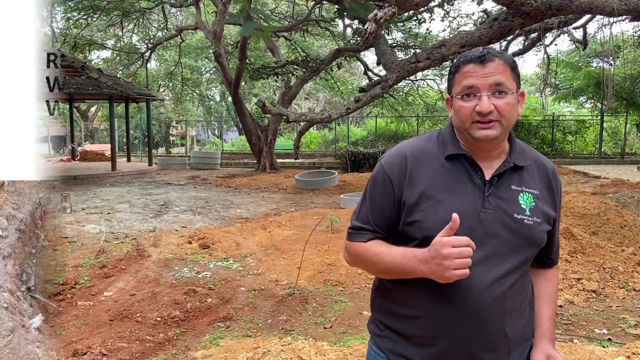 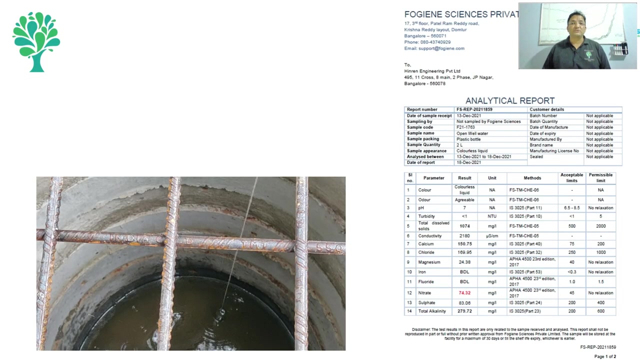 So now we will try to sample this water from the well and send this for testing and see the quality of the unconfined aquifer or the shallow aquifer. So we just saw in the field The borewell and the recharge well we also found that there is water in the recharge. 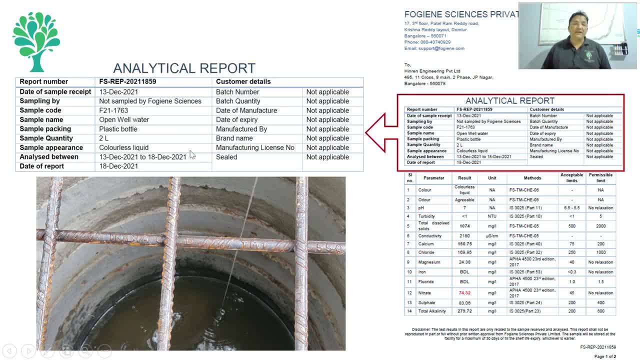 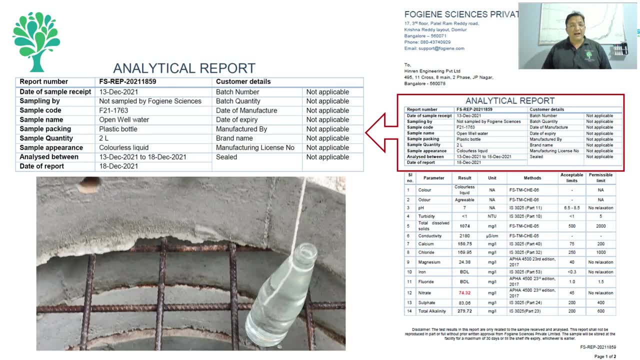 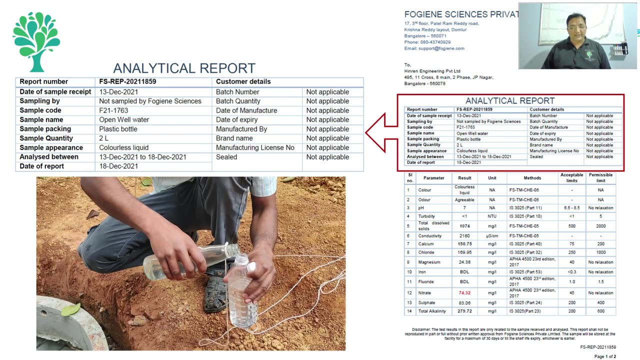 well, We sent this water for testing and this water was sampled on the 13th December and it was sent for testing to test under is 10: 0, 5 double 0 drinking water standards. Now let us quickly run through this test report and see what best this water can be used for. 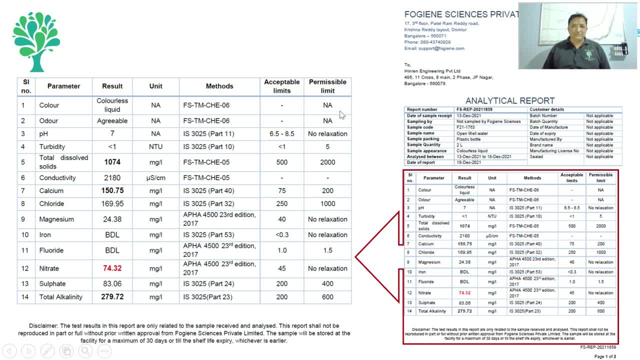 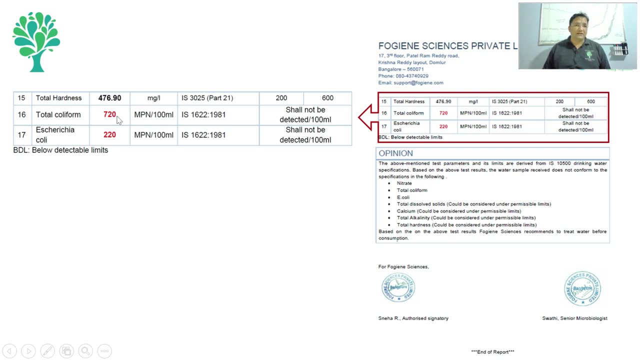 This is the test report. all physical parameters seems to be okay. However, in chemical parameters the TDA seems to be higher. calcium also seems to be higher, nitrate is definitely much on the higher side and if we look at the biological parameters, the total coliform and Ecoli both seems to be very much on the higher side. 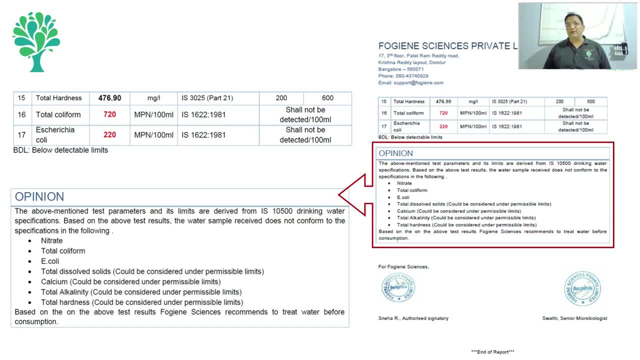 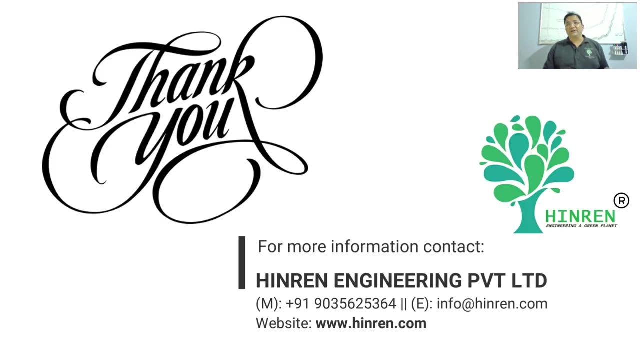 So this water technically doesn't doesn't fit for drinking. However, this water can definitely be used for any kinds of non-portable purposes, like gardening, landscaping, Carving, Water wash or any other kinds of non-portable use. So thank you very much. 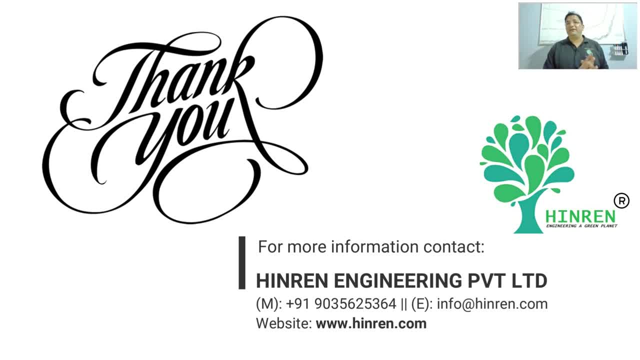 So in just the shallow aquifer, needs to be explored and studied much more in detail. The water available at shallow depths are definitely good in terms of quality and also perhaps the water available at that shallow depth is the cheapest source of water. I have done another exclusive video on the economics of this recharge wells. 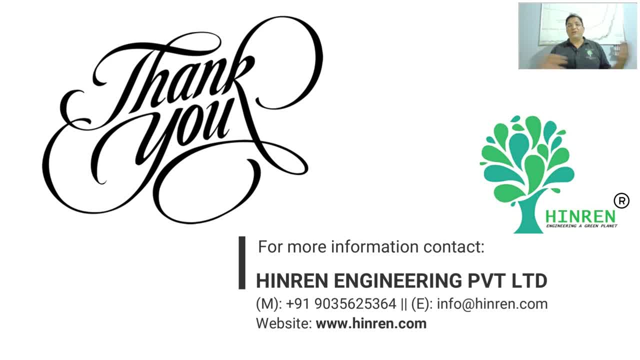 The link is in the description, So I would urge people to actually look at shallow aquifer as a source of water. So thank you very much.